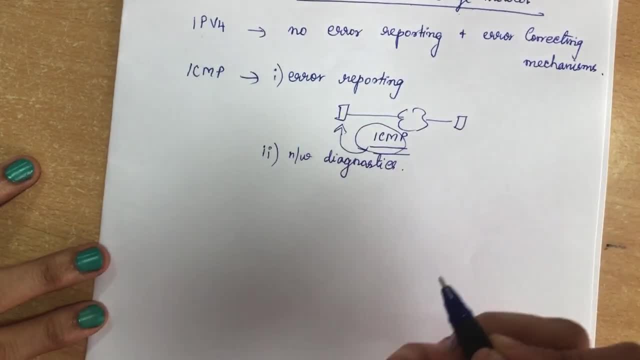 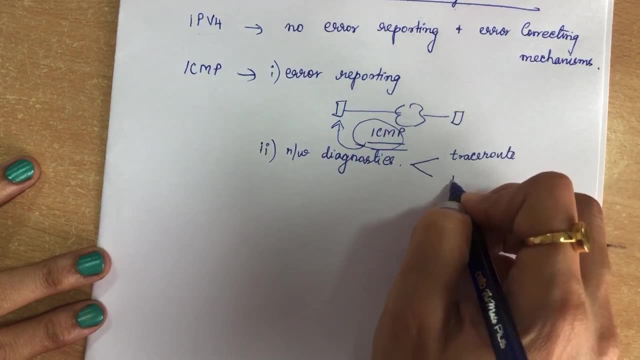 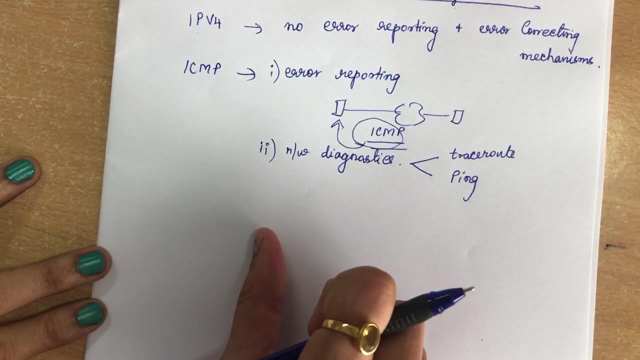 Okay, the common, the commonly used network diagnostics are trace root and the second one is ping command. ARE TRACE ROOT, TRACE ROOT, TRACE ROOT, ping command? okay, what is the use of this? trace routers? so trace route will display the routing path between the two devices, between two internet devices. it will tell. 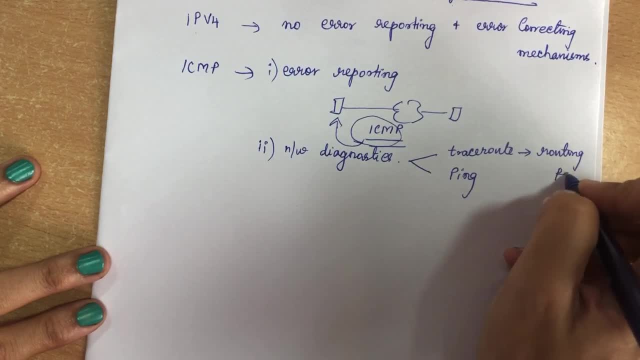 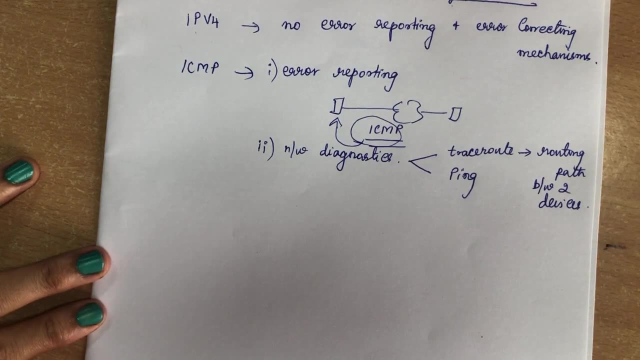 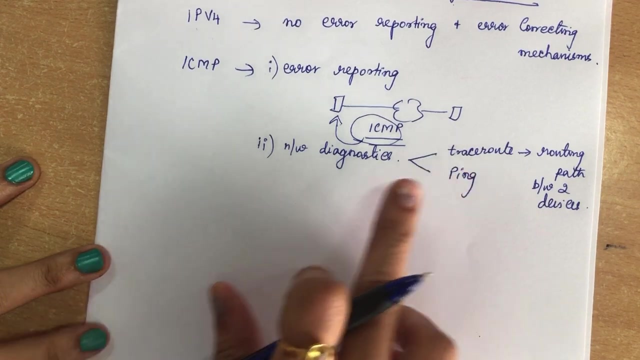 you the routing path? okay, this routing path, it is nothing, but it's an actual path between the two connected devices. okay, this is the trace route. okay, and what is ping? ping is also a simplified version of trace route. what this will do is you can test the speed. 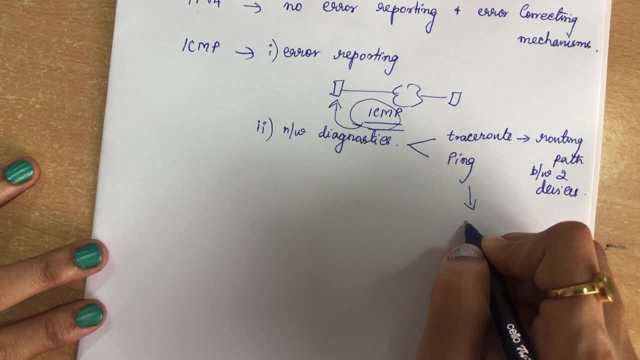 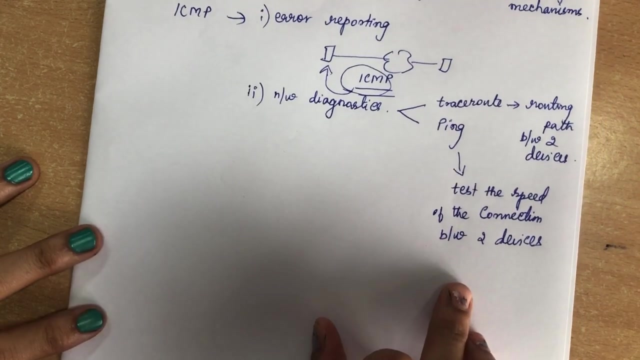 of the connection between the two devices. using ping command, you can test the speed of the connection. test the speed of the connection between the two devices, and it will also report exactly How long it takes a packet of data to reach its destination. okay, and come back to the 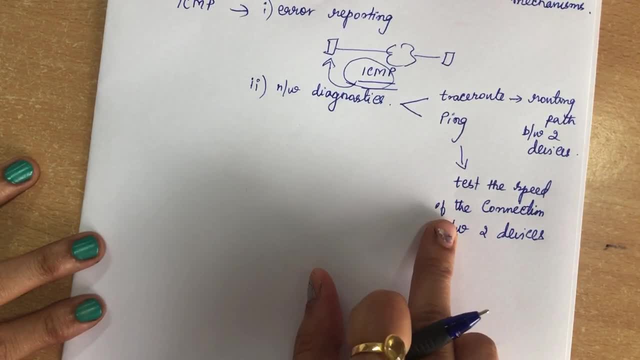 sender device. so this ping command is used to test the speed of the connection between the devices and it will also report. that is like. it will also tell how long a packet will take to reach the destination and come back to the sender. so these are the primary. 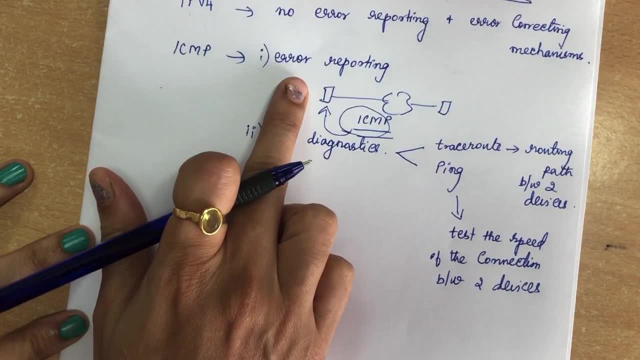 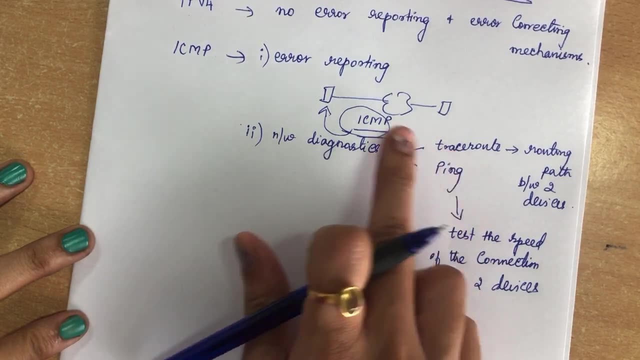 functions: primary and secondary functions of ICMP. the first is reporting error messages to the sender device. the second is used to used as a diagnostic tool. Okay, To find out to do these two functions, which will have two functions. one is trace route. 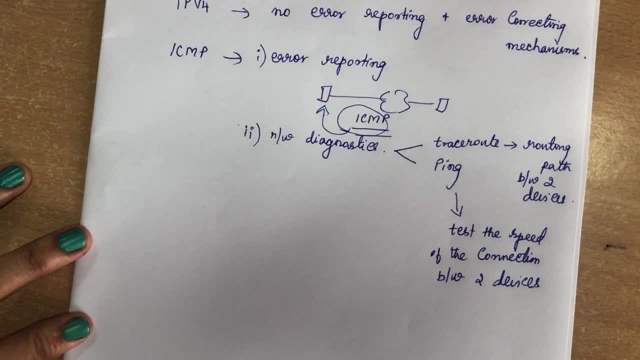 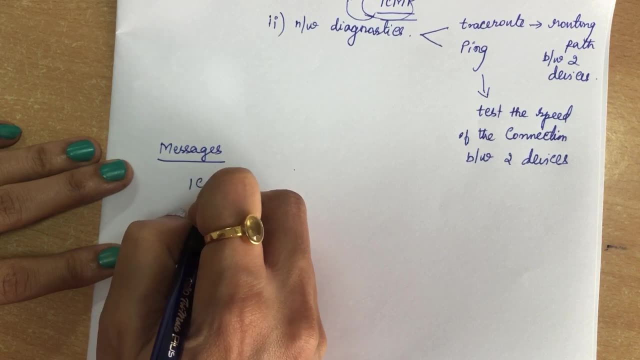 other one is ping command. so we will see in detail on error reporting now. So next coming to the messages. okay, so coming to the first error reporting messages. so again this ICMP messages, it is divided into two categories. okay, it is divided into two. 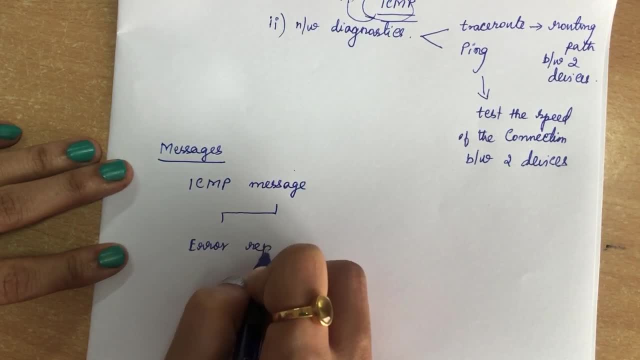 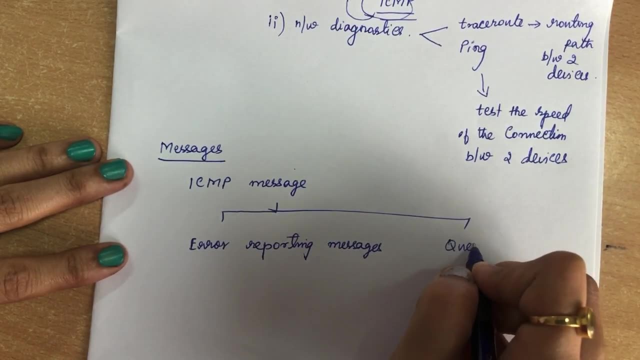 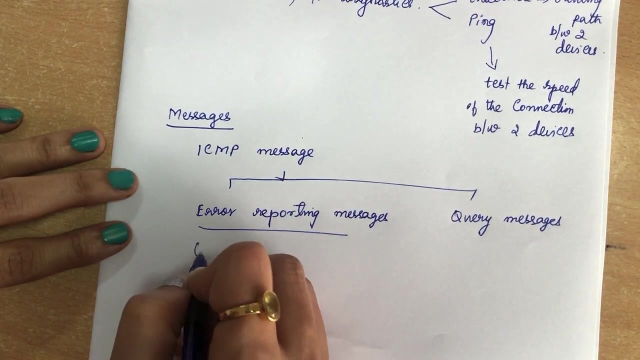 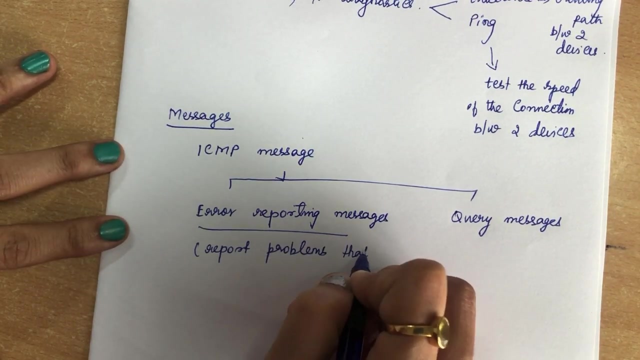 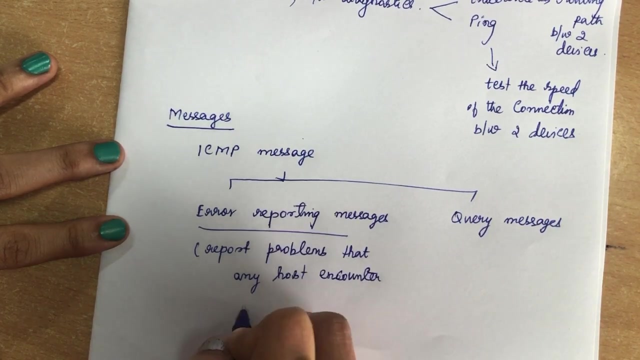 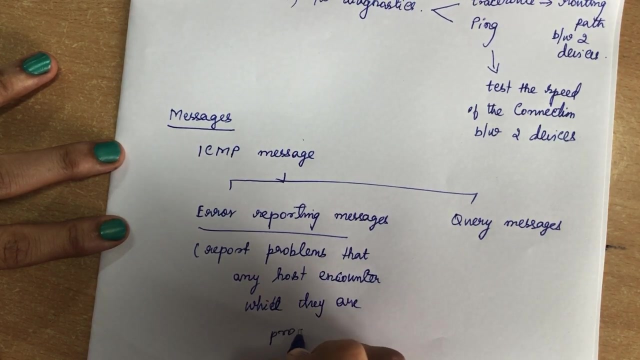 categories. one is error reporting messages and second one is query messages. So what does this error reporting messages will do? This will report the problems. report problems that any host encounter, or any router or encounter while they are processing the packet. while they are processing the packet, okay. 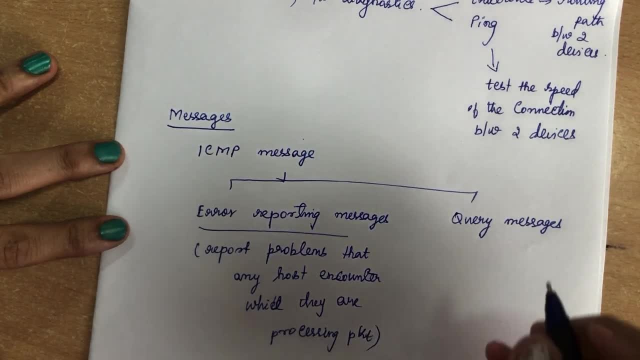 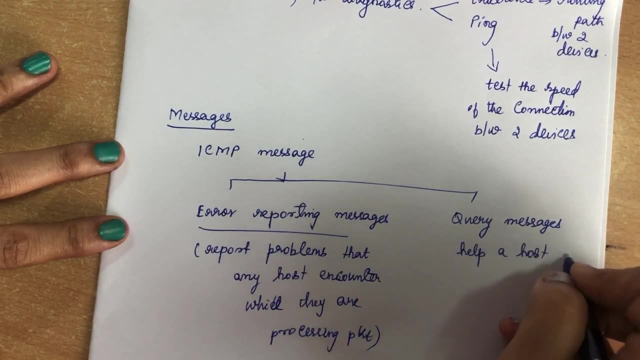 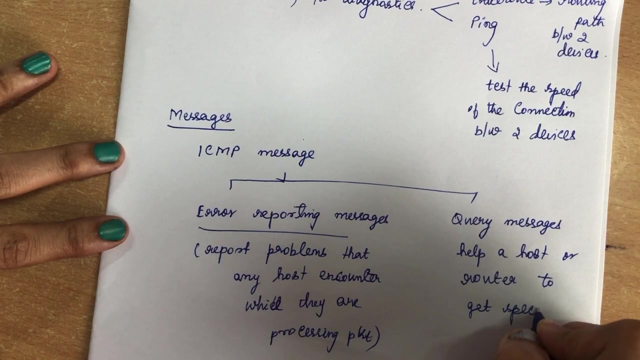 Okay, And what is this? query messages. The query messages: nothing, but it will help a host or any router to get specific information, to get specific information about another host. So there are two messages it will handle ICMP. one is error reporting and query error. 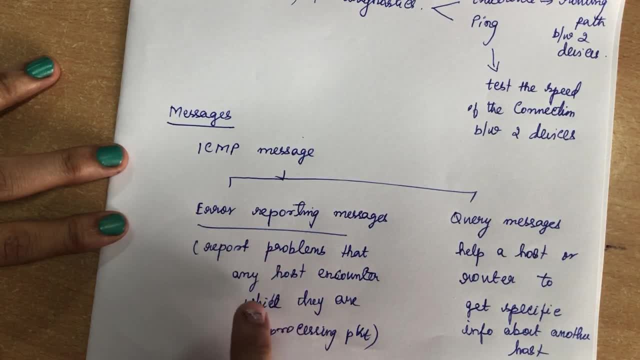 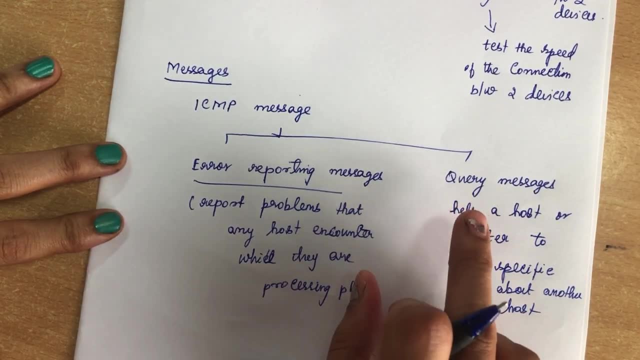 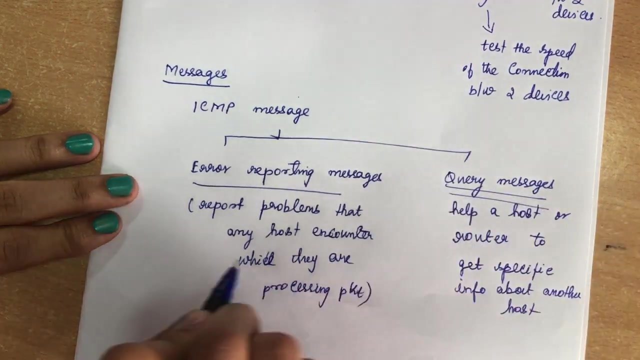 reporting will tell you. it will report the problems whenever any host. that is like whenever any host encounters while they are processing the packet- but query messages, it will helps any host to identify or to know about any other information about any other host. so that is, using query messages we can able to find out. okay, these are all about ICMP messages. 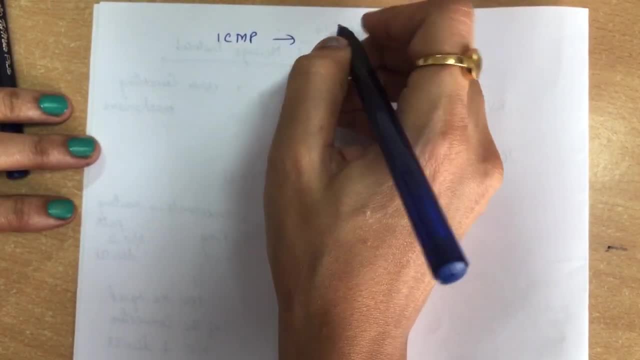 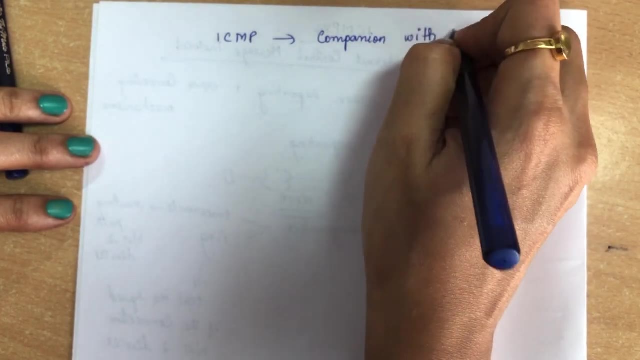 ICMP protocol. it will not work in separate. okay, it will always work in companion with IP protocol. It works companion with IP protocol. Okay, How does it work? is like it will. here. we are not going to send it directly to the data. 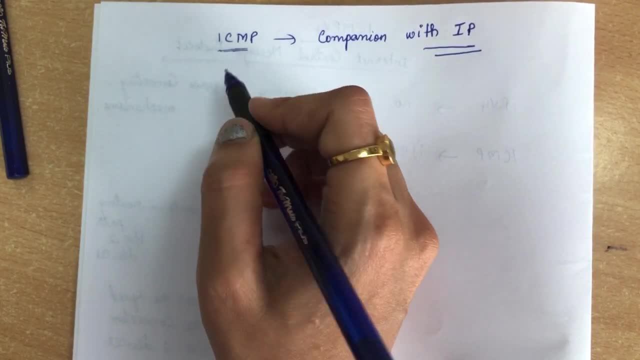 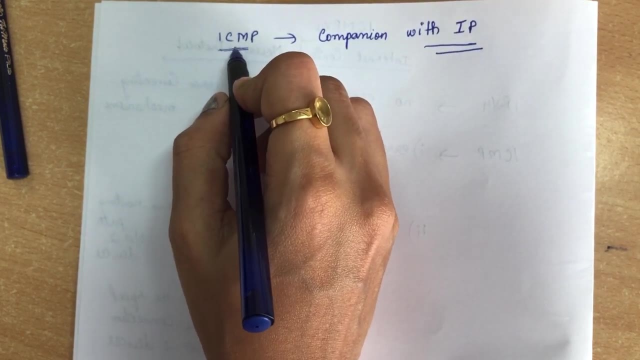 link layer. ICMP protocol will not send any data directly to the data link layer. it always work in companion with internet protocol. So whenever a messages, whenever you have error messages, that will be that is, that will be encapsulated along with IP datagram. 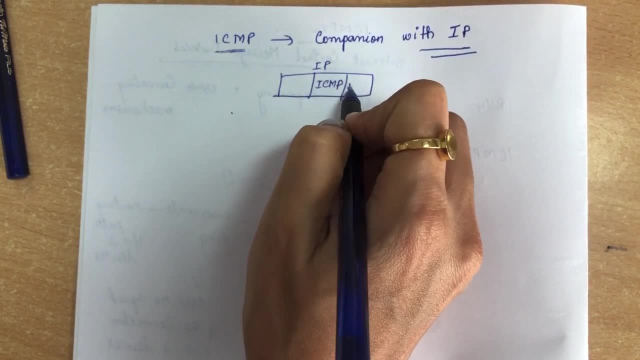 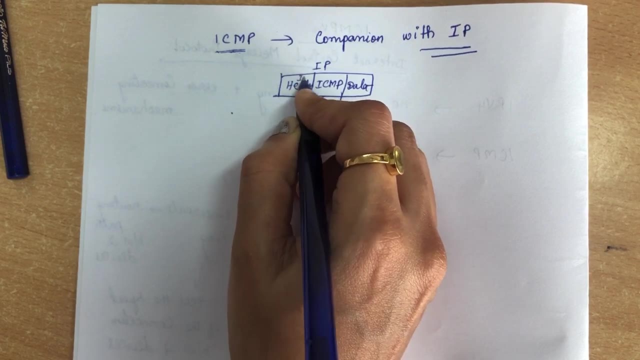 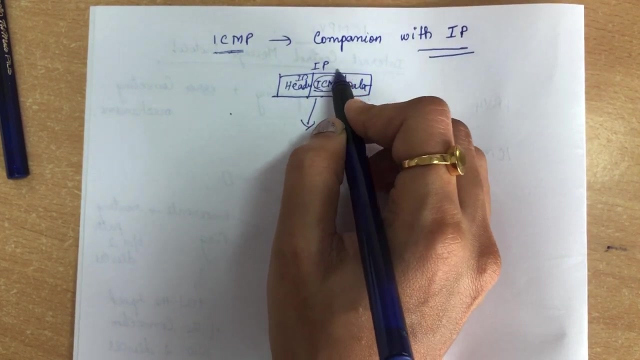 So first, ICMP messages will be. you have a data and this ICMP messages will be encapsulated and again this IP header. it will be there. IP header will be there. then that messages will be sent to the data link layer. So when it is mentioned over here, when it is added internet protocol as to specify the 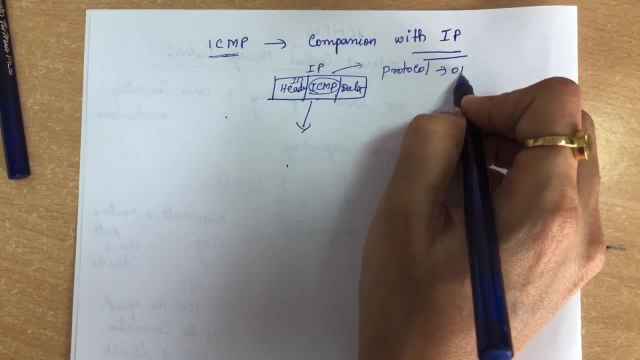 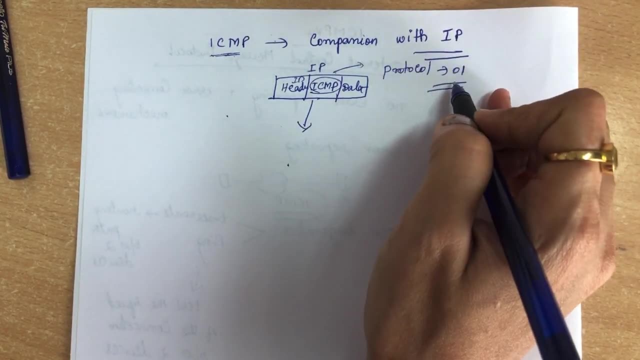 protocol value to be protocol value to be 01,. as we have already seen in internet protocol that suppose if ICMP protocol is also used along with IP, then the protocol value is 01, that we have to mention it in the header IP, IP header. 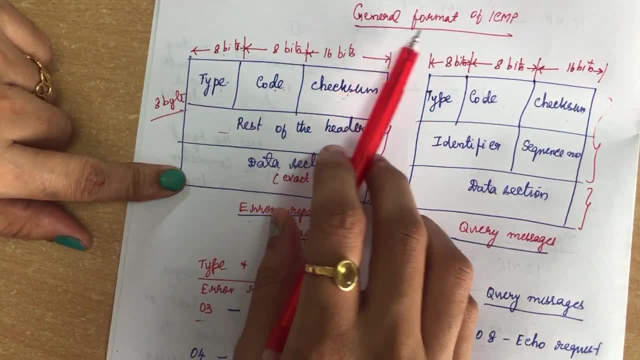 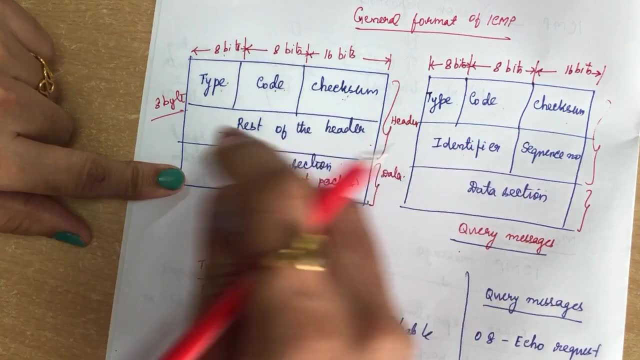 Okay, Next comes a general format of ICMP. Coming to the general format, it will have an header part and then it will have the data part over here. Okay, Header part is of 8 bytes and remaining section. we have the data part. 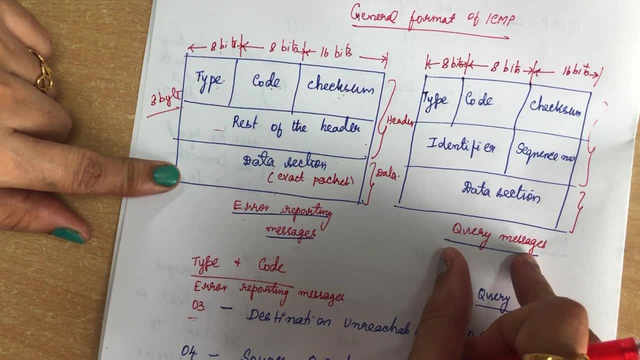 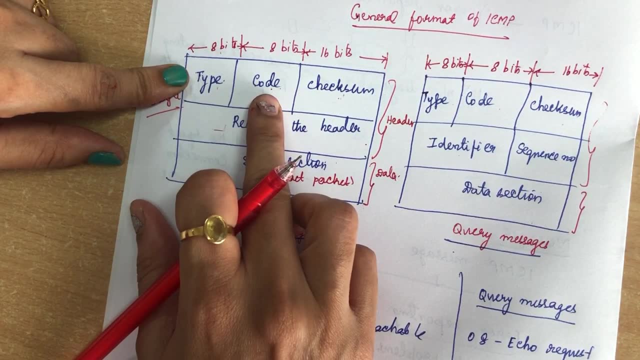 So likewise we have for error reporting and then for query messages. Okay, So coming to the header part, it contains a type type of the error message code, the reason for which the message, reason for the message type and the checksum value will contain. 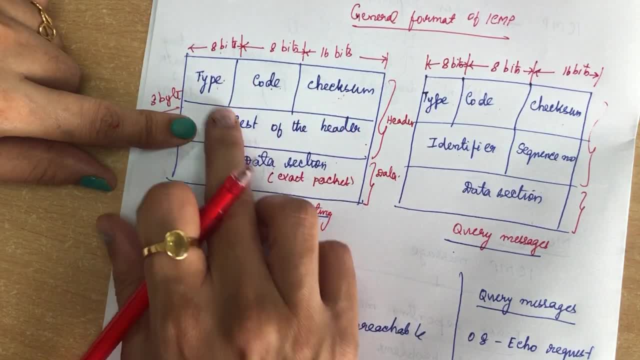 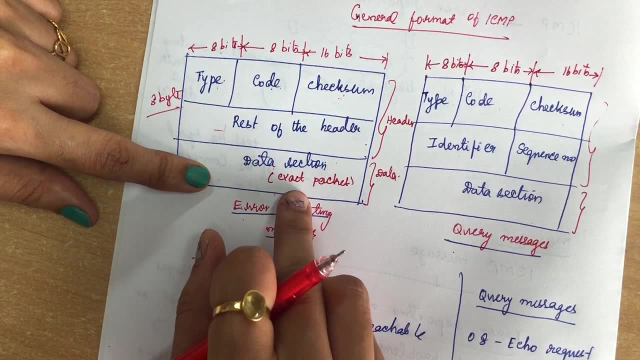 will helps for error correction Or error reduction, and then the rest of the header. So next is data section. This data section contains information about the exact packet that had the error. Okay, Coming to this query message, also the type of the error, type of the query message and 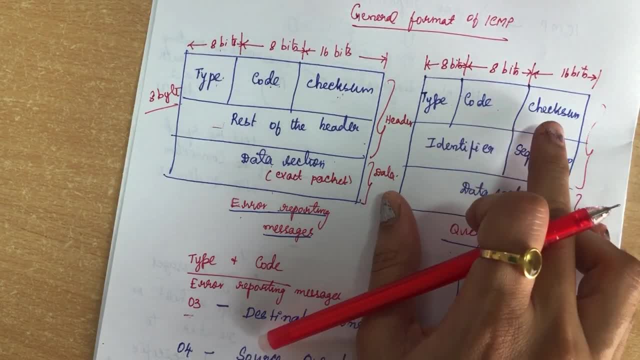 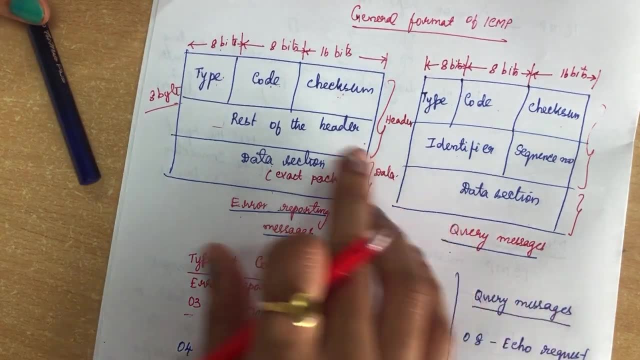 what is the code value will tell you the reason for that particular message type, and then checksum value. You have an identifier for identifying the query message and the sequence number and the remaining data section. Okay, This is all about your this ICMP. So, coming to this type, 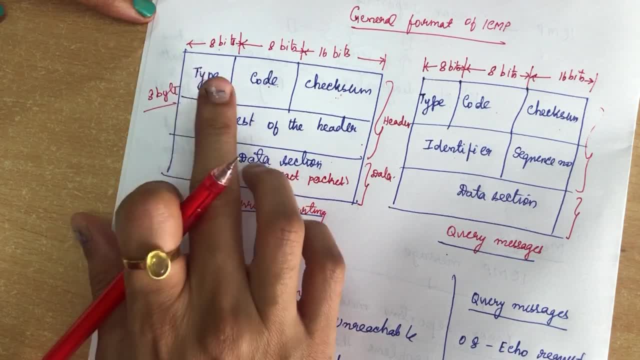 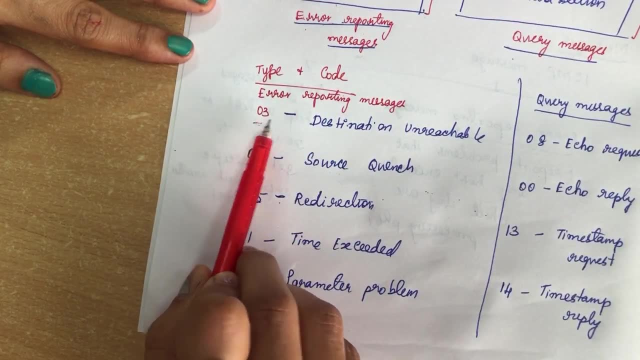 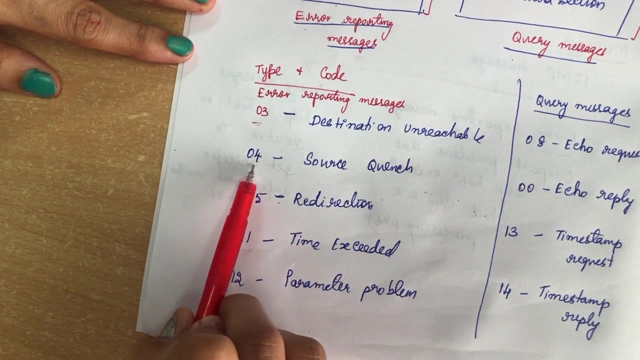 So there are several types are available, but commonly used types only we will discuss here. So, coming to the type and code of this error reporting, we have 03.. So when the destination is unreachable, then ICMP will send a report message called error reporting, message, called 03, and you have the next value, 04, the type of the value you can. 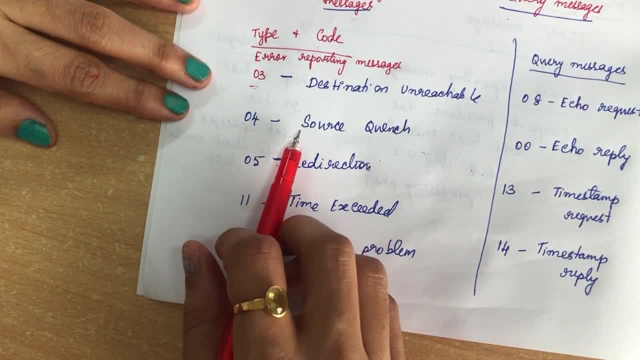 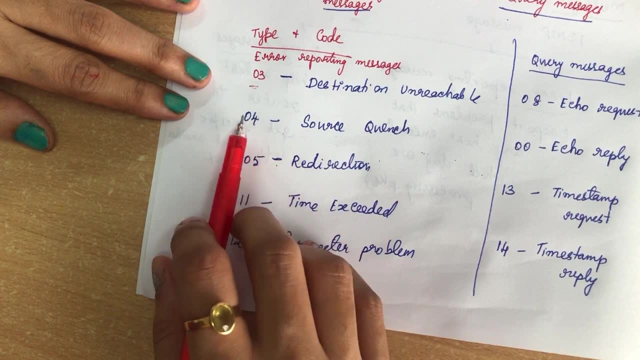 have the 04.. What does this 04 will tell you, is when source is overwhelming the path, then some of the packets will get lost. So ICMP will. what it will do is it will send 04 message to the source saying that source. 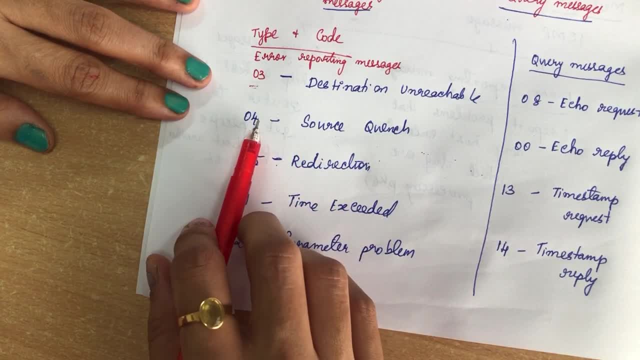 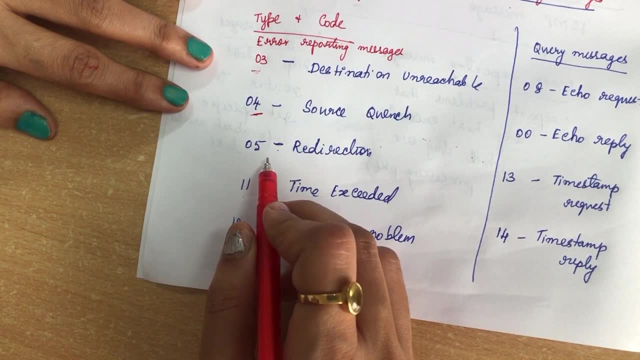 quenched, It has to reduce the flow control. That is why it is sending this error message to the sender. Okay, Next is redirection. Redirection- how it will work- is data whenever you want to send the data to the. that is. 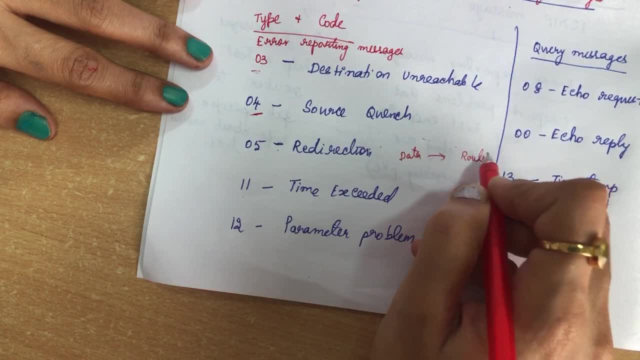 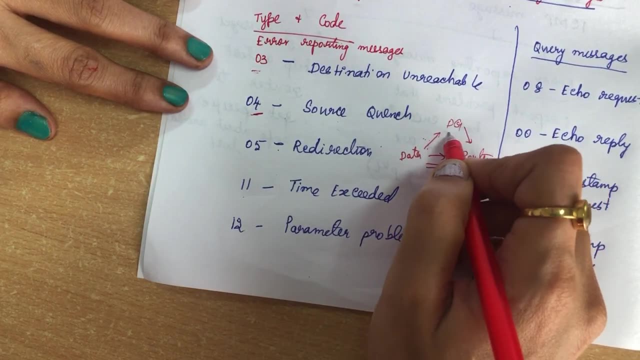 like whenever a source wants to send the data to the router through that path. so it doesn't find the path to the router. So what happens is we will find we have a default gate. Okay, We have a default gateway, So we will send a packet to the default gateway. 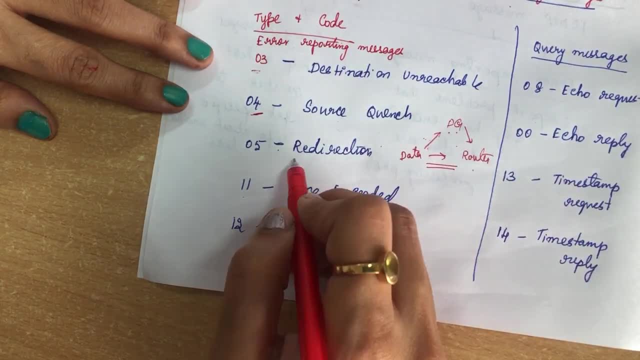 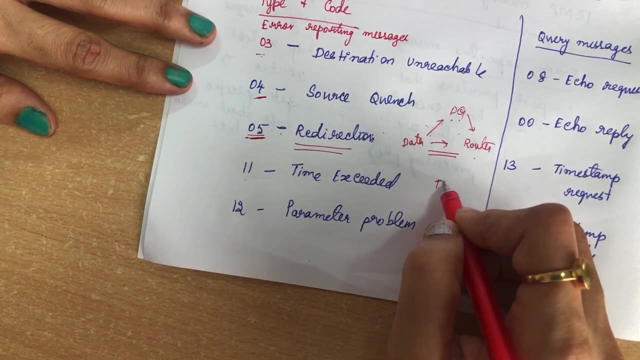 From that default gateway it is, it will be sending to the router. So in that case redirection will be used, So you have to use the code called 05.. Next is time exceeded. So when time to live value? usually whenever the sender it sends a packet, it will it. 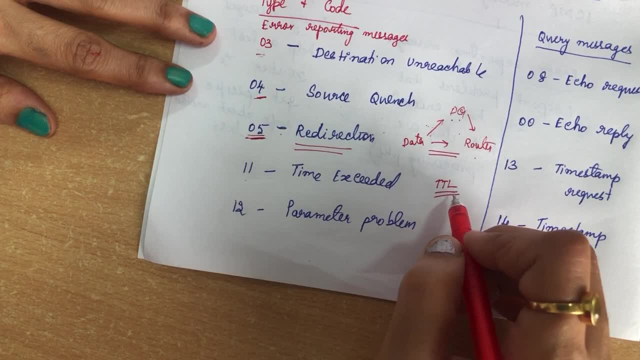 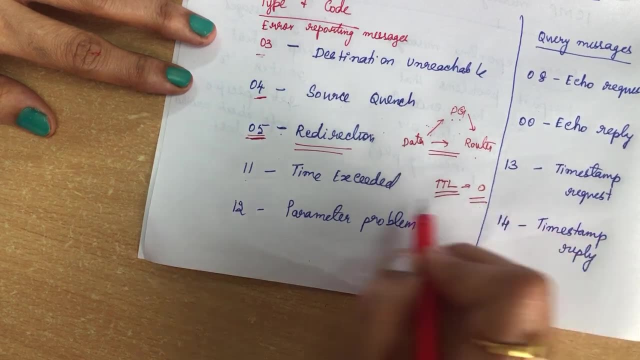 will set some TTL value. This value will be decremented whenever this packet reaches any host or in between routers, So whenever this TTL value becomes zero. So this ICMP packet, This ICMP packet will send a message 11 to the sender saying that the TTL, the time has. 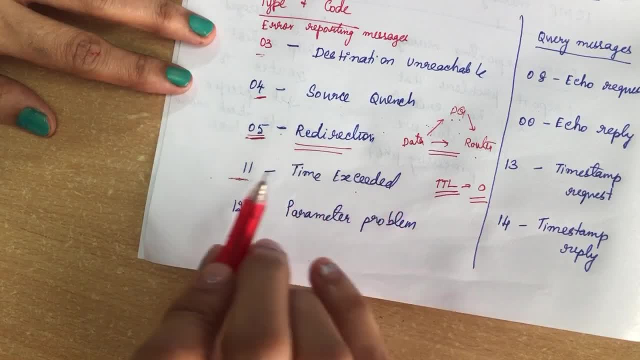 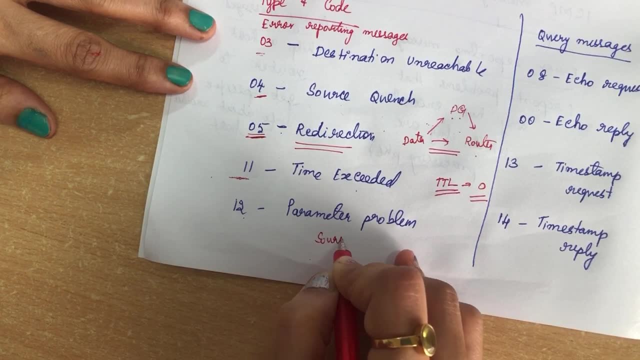 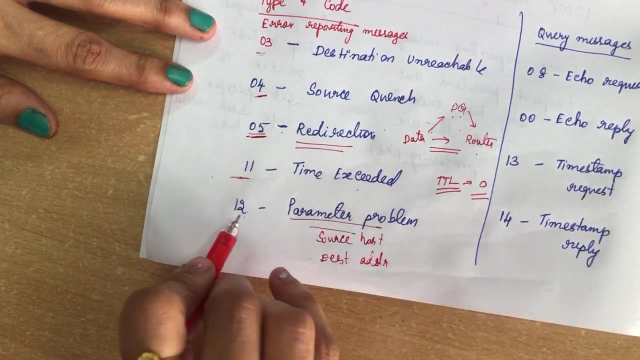 exceeded. So it has, it has to, it has discarded the packet, So this is 11.. Next is 12.. So when any parameter, like source, like source host, host address or otherwise destination address- is missing, then the parameter problem is missing. then this 12 message, 12 value. 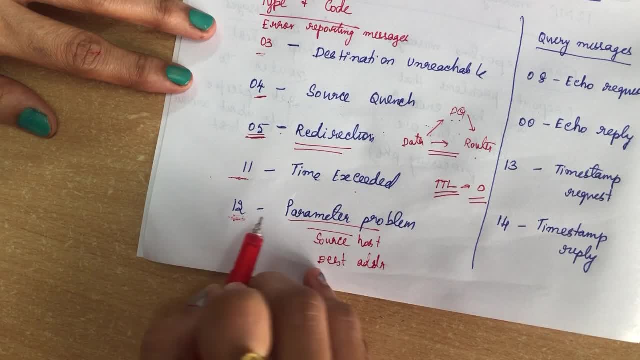 will be used. 12 value is used to say that any of the parameters are missing. Okay, Okay, So we will use the code. We will use the code to say that any of the parameters are missing in your data set. Okay. 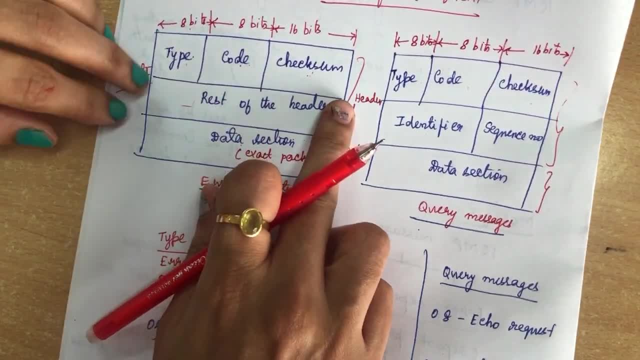 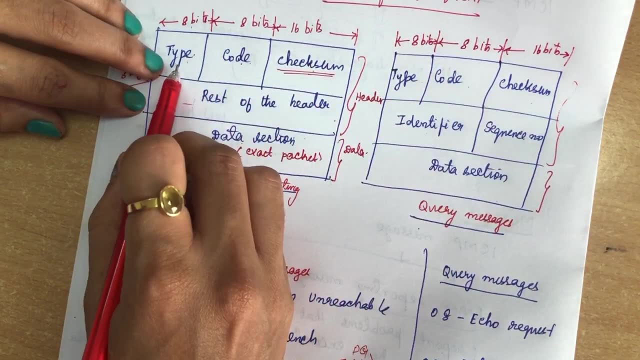 This is a header part, So these are all the type and code of your the error reporting messages. What is the use of checksum value? Checksum value: How it will be calculated. this, So you will have all the values for this. 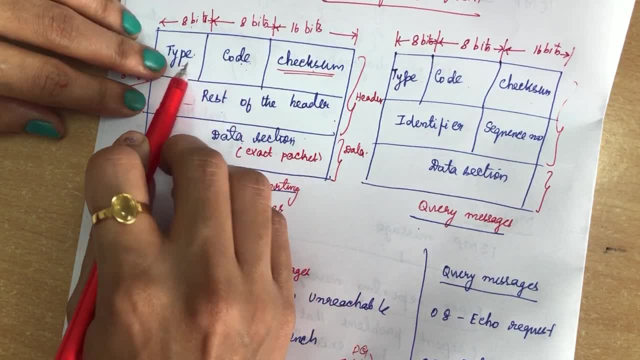 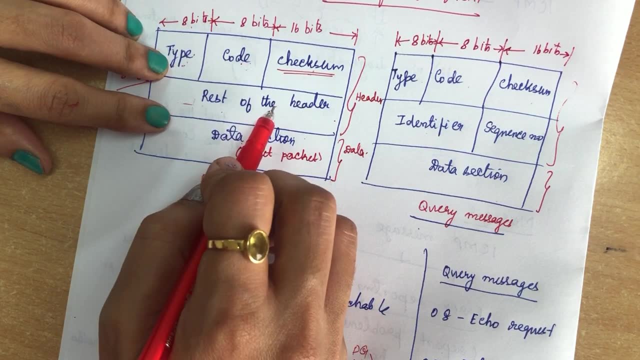 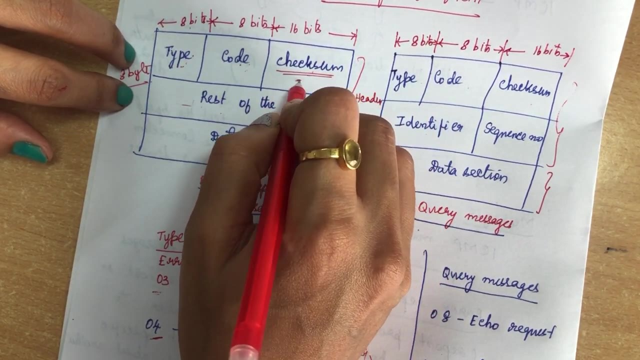 So whenever we are sending the data, we will add all the type, type, value, code, value and the headers over here and the data. after adding everything we will do, the once compliment of that summation We will get the final result. final result will be considered as checksum. we will send it through the header, so in the receiver. 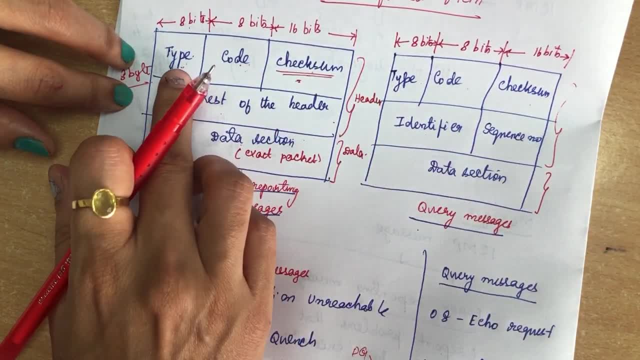 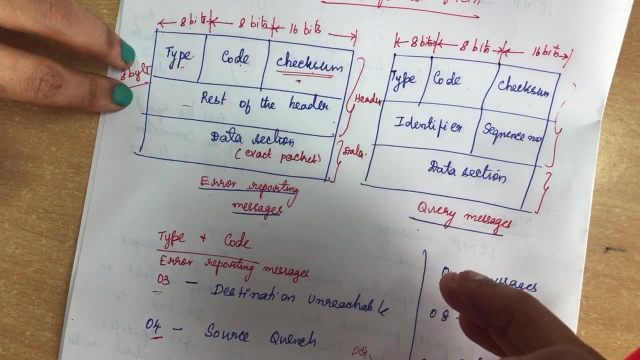 what they will do is they will take this checksum value and likewise they will also add all the values inside your header and data part and they will find out the sum. that sum they will be doing once complement. so when they do that, that value should be same as checksum value, if both are same.